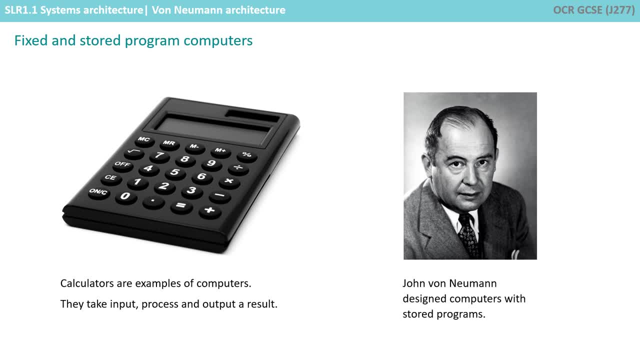 program computer. It can do mathematics, but it cannot be used for any other purpose. Changing a program of a fixed program machine requires rewiring or redesigning the machine. A stored program computer is one that has changeable programs. In 1945 the mathematician and physicist John von Neumann described the 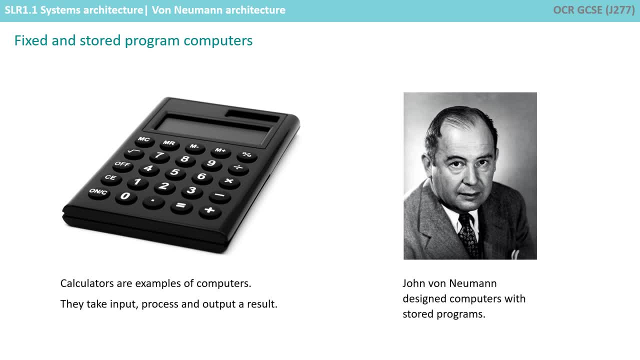 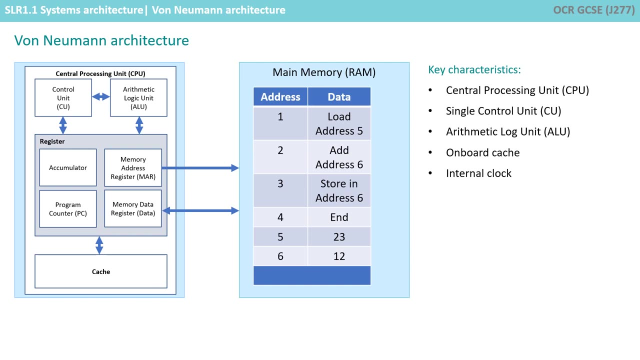 first design for modern computers that had stored programs. This way of designing computers became more popular, known as the von Neumann architecture. a von Neumann architecture has key characteristics: it has a central processing unit, a CPU, with a single control unit inside. it has an arithmetic logic unit, an ALU onboard cache, which is 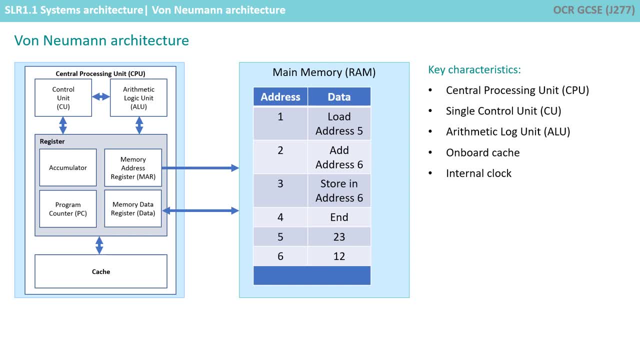 small amounts of high-speed memory that helps the control of instructions and data around the CPU, and also an internal clock which provides a pulse at a constant rate to synchronize components. this architecture computer fetches, decodes and executes instructions. this isn't the most efficient design for 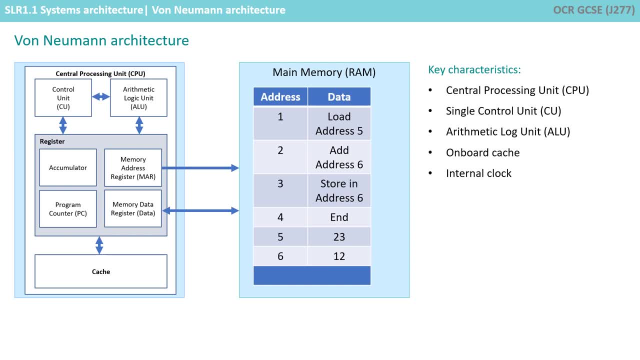 processing. but it was indeed simple. programs are made up of a sequence of instructions stored in the main memory outside of the CPU. they're fetched one by one to the registers for processing. let's have a closer look at the memory. you will notice that each instruction is stored in a location in the memory and 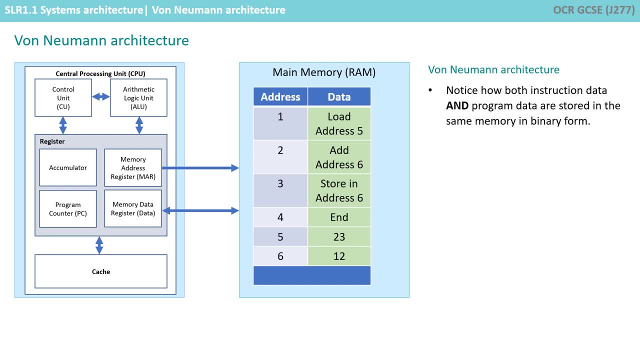 each location has an address. therefore, the processor can fetch an instruction stored in memory address one for example- and bring it back into the processor. now, computers are complex machines capable of fetching and executing instructions billions of times a second, using a very methodical sequence of events inside the 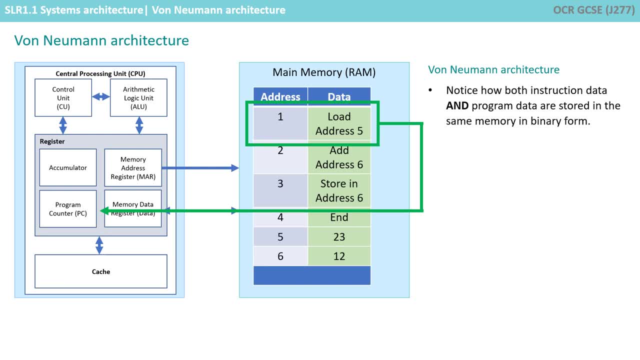 memory. in order to do this, they make use of special-purpose registers, which we introduced in the last video. let's take a look at each one and see what it's used for. the program counter always holds the memory address of the next instruction to be executed. once we fetch this address from the program counter, we 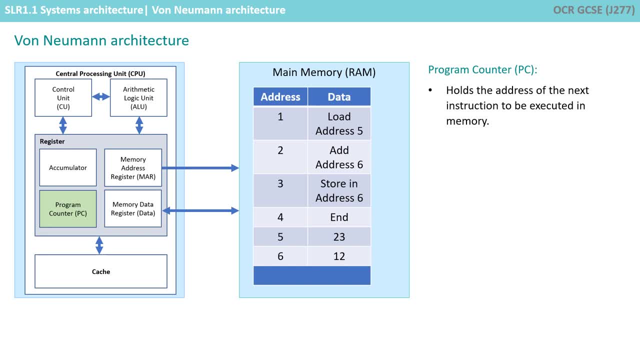 increment its contents by one, so it points to the next instruction to be executed. the memory address register holds the address of where data is to be fetched from or stored into the memory. data register holds any data which has been fetched from memory or is about to be written to memory. the accumulator holds: 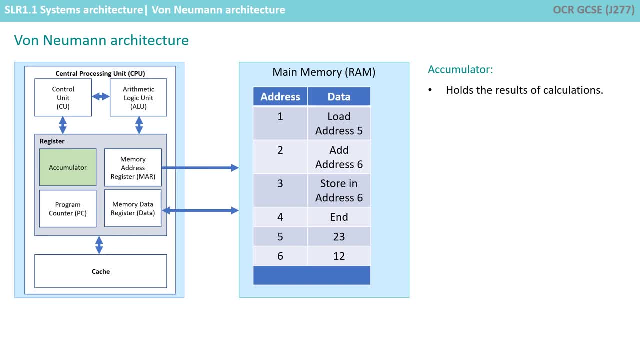 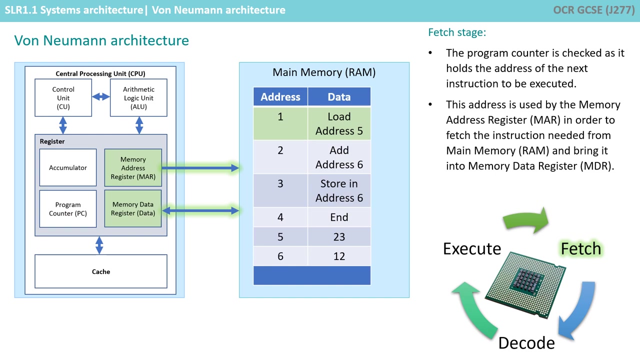 the results of calculations which have been performed by the arithmetic logic unit. let's look at a typical fetch execute cycle in a little more detail. so we start with the fetch stage. the program counter is checked as it holds the address of the next instruction to be executed. this address is used by the memory address register. 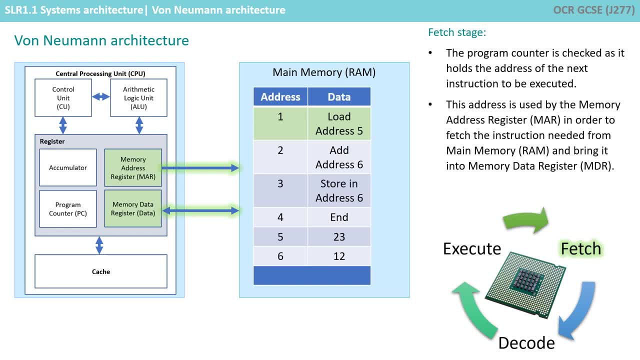 in order to fetch the instruction needed from main memory and bring it back into the memory data register, the address in the program counter is incremented to point to the next instruction. now the instruction is in the CPU. the control unit decodes the instruction to see what has to be done. 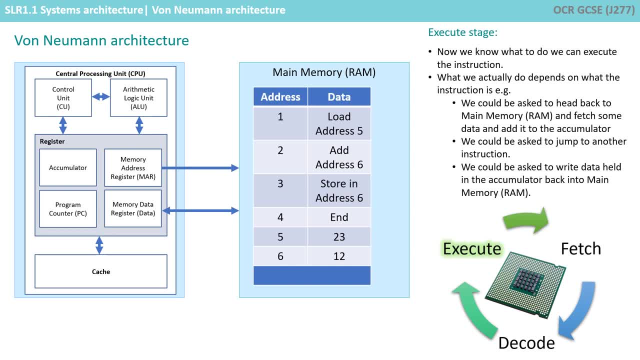 now we know what to do. we can execute the instruction. what we actually do depends on what the instruction actually is. we could be asked to head back to main memory and fetch some data and add it to the accumulator. we could be asked to jump to another instruction. 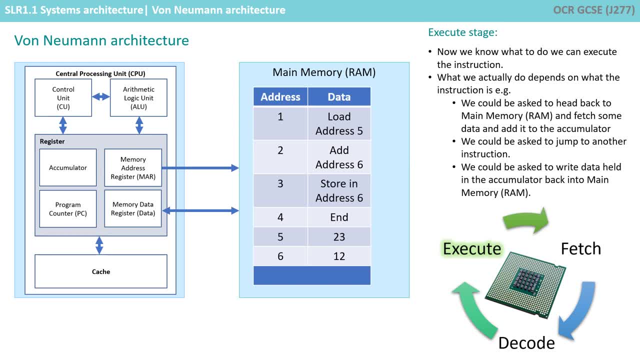 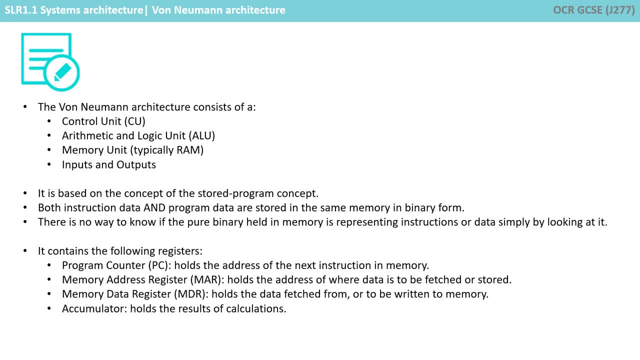 so we can execute the instruction and bring it back into the memory data register. we could be asked to write data held in the accumulator back into RAM. so let's just recap what we've covered so far. the Von Neumann architecture consists of a control unit, an arithmetic logic unit, memory unit and inputs and outputs. it is 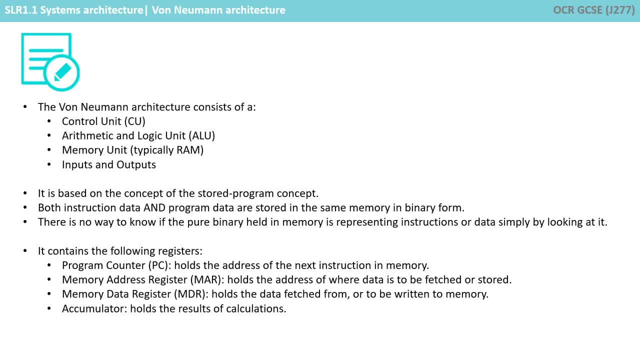 based on the concept of the stored program concept. both instructions data and program data are stored in the same memory in binary form. there is no way to know if the pure binary held in memory is representing instructions or data, simply by looking at it. it has to be brought into the. 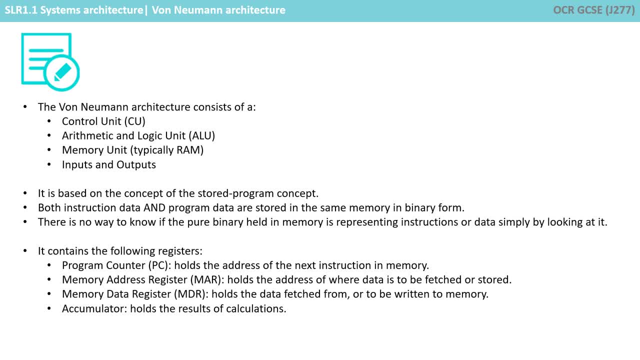 processor and decoded, and it contains the following registers: the program counter holding the address of the next instruction to be executed in memory. the memory address register holding the address of where date is to be fetched or stored. the memory data register holding the data fetched from or to be. 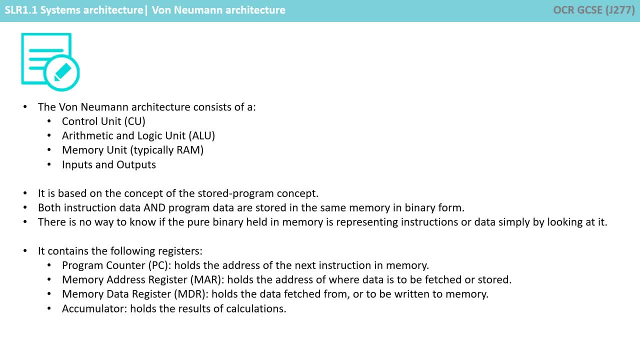 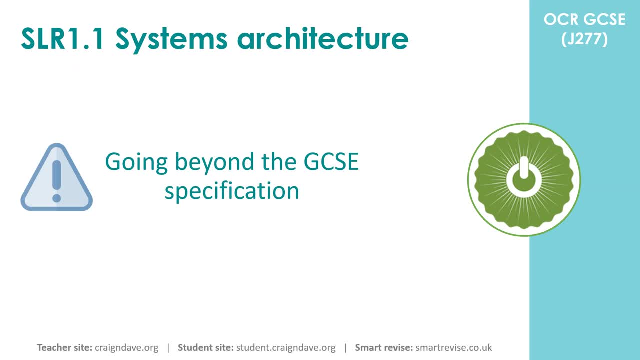 written to memory and the accumulator holding the result of calculations. What comes next is technically a little beyond what you need to know for the GCSE exam, so there's no need to take notes on the rest of this video. However, if you're looking for a slightly deeper level of understanding, this next section will 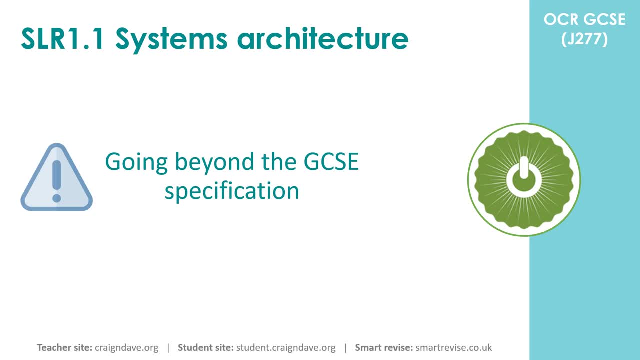 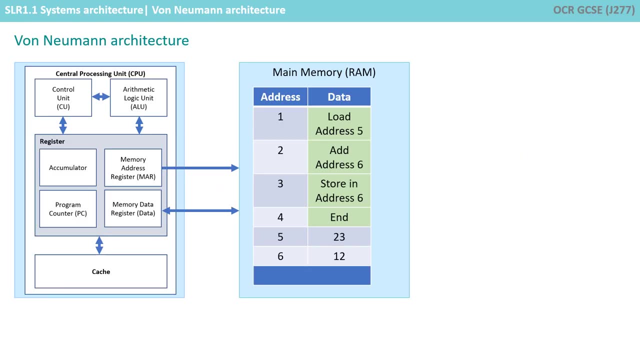 really help bring together everything we've covered in the last three videos and excellent bridging knowledge for the A level. So in the final section of this video we're going to follow through the various stages of the fetch execute cycle to see exactly how the program instructions stored in memory locations. 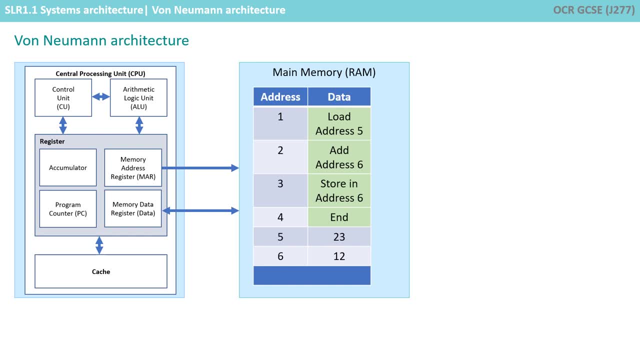 1 through 4 are carried out in the CPU. So we start with the fetch cycle. The program counter is checked as it holds the address of the next instruction to be executed. The address is copied into the memory address register. The address goes down. 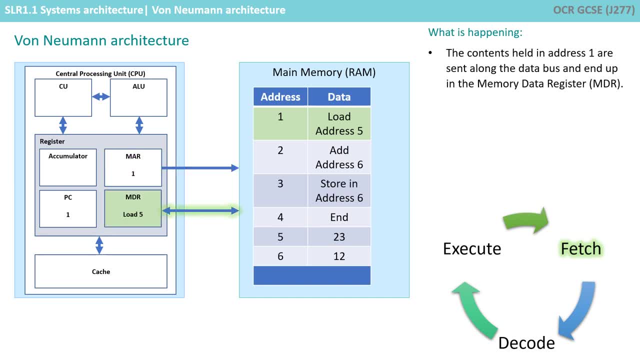 the address bus and the contents held in address 1 are sent along the data bus and end up in the memory data register. So that was the contents load address 5 and you can see that's come back and it's now inside the MDR. 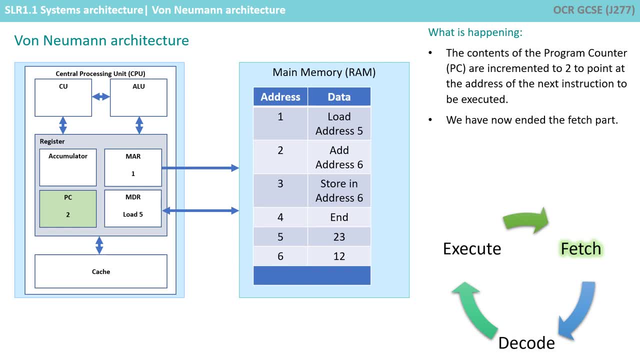 The contents of the program counter are incremented to 2 to point at the address the next instruction, and we've now ended FETCH. Now we're on DECODE. The first thing we do is take a copy of what's just been loaded into the CPU and place it into the cache. This means if 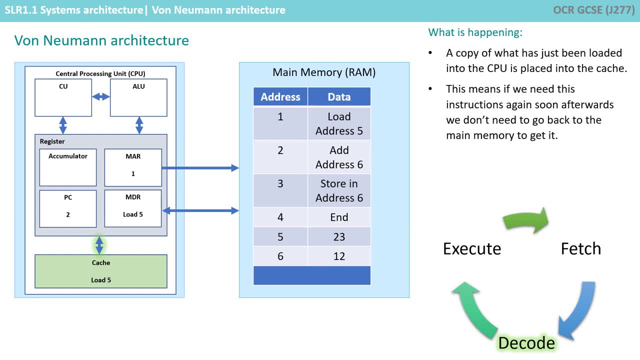 we need this instruction again soon afterwards. we don't need to go back to main memory to get it. The control unit now decodes the instruction, that's LOAD5.. It discovers it needs to load the contents which are stored in memory address 5, so we update the memory address register with. 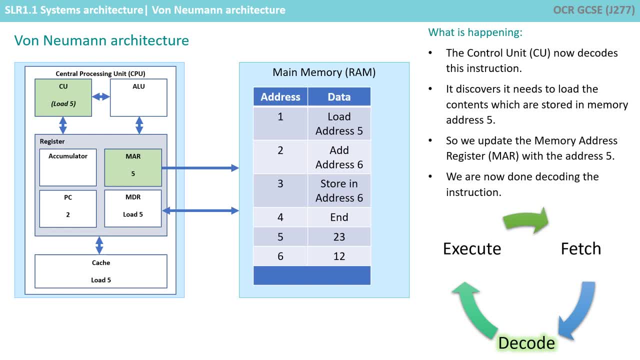 address 5.. We're now done decoding the instruction. We now execute the instruction and so pass address 5 down the address bus. We then return the contents of address 5, which is the value 23, down the data bus and place it into. 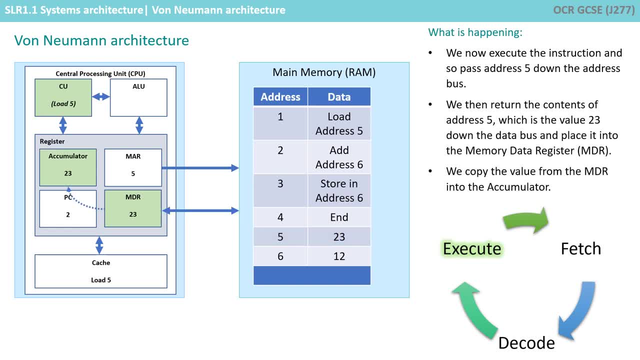 the memory data register. We copy the value from the memory data register into the accumulator. A copy of the value 23 is again placed in the cache in case it's needed again. Note that although the contents of the registers are being overridden, the functions are that they are normally larger and so can hold multiple items. 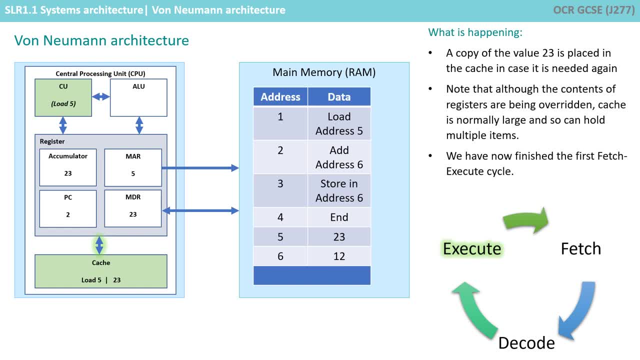 We have now finished our first FETCH execute cycle, So we're on to the next And of course we start with FETCH. The program channel is checked as it holds the address of the next instruction to be executed. The address is copied into the memory address register. 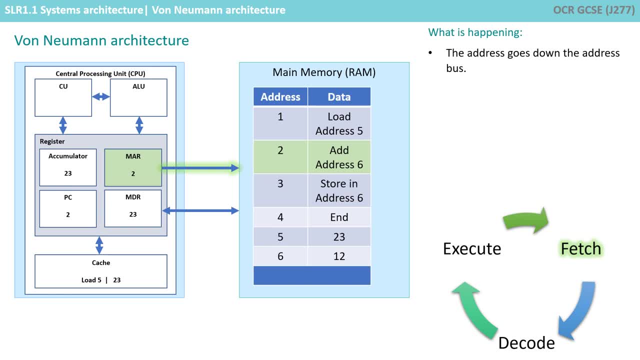 The address goes down the address bus 2 are sent along the data bus and end up in the memory data register. So this time it's the content add address 6 that's ended up back in the MDR. The contents, the program counter are incremented from 2 to 3 to point to the address of the next. 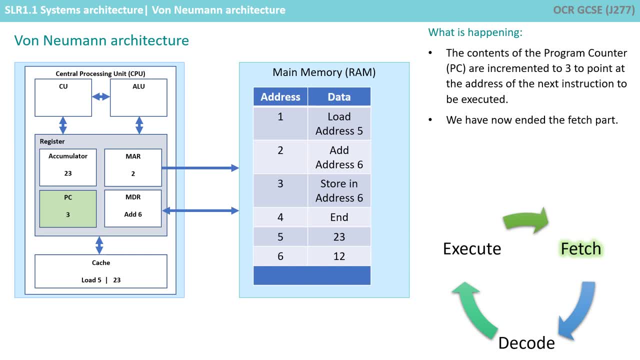 instruction to be executed. We've now ended the fetch part. Again, a copy of what's just been loaded in the CPU is placed into the cache. The control unit now decodes this instruction, add 6.. It discovers it needs to add the contents. 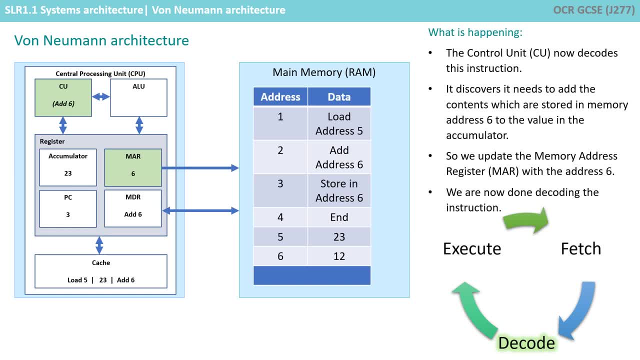 which are stored in memory address 6 to the value we currently have in the accumulator, which is 23.. So we update the memory address register with address 6.. We're now done decoding the instruction. We We now execute the instruction and so pass address 6 down the address bus. 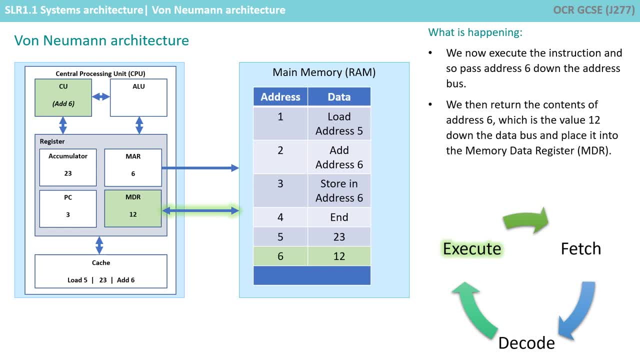 We then return the contents of address 6, which is the value 12, down the data bus and place it into the memory data register. We store a copy of the value 12 in the cache in case we might need it again soon. 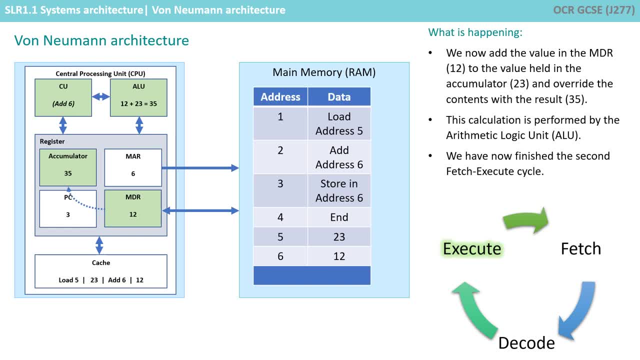 We now add the value in the memory data register, that's 12,, to the value held in the accumulator, which is 23,, and we override the contents with the result 35.. This calculation is performed by the arithmetic logic unit. 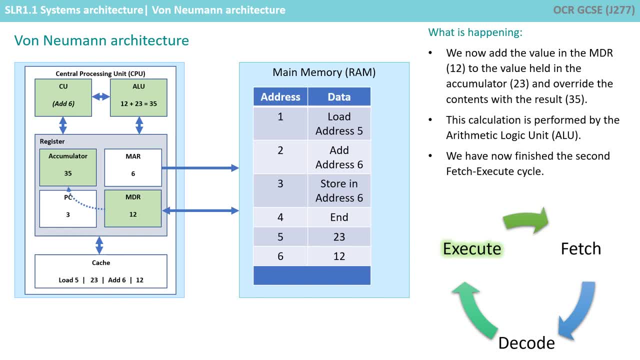 We've now finished the second fetch execute cycle and it's time to start the third. The program counter is checked as it holds the address of the next instruction to be executed. The address is copied into the memory address register. The address goes down the address bus. 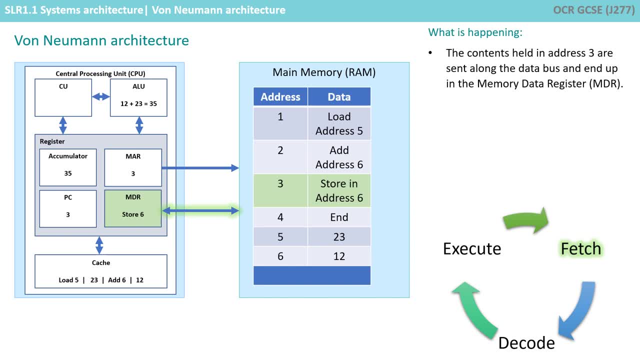 The contents held in address 3 are sent along the data bus and end up in the memory data register. The contents the program counter are again incremented to 4, this time to appoint the address of the next instruction to be executed Again. we've now ended the fetch part. 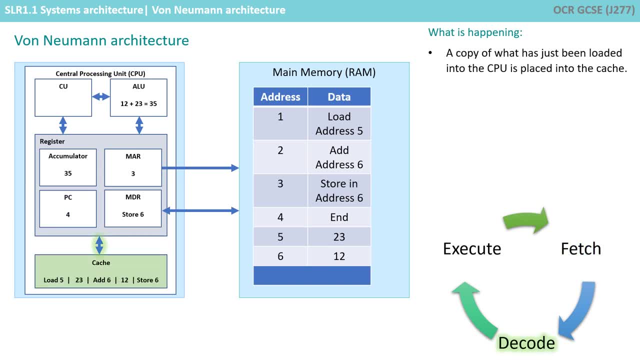 A copy of what's just been loaded into the CPU is again placed in the cache. The control unit now decodes the instruction. We discover we need to store the contents of the accumulator into memory address 6.. So we update the memory address register with the address 6 and we copy the value in the 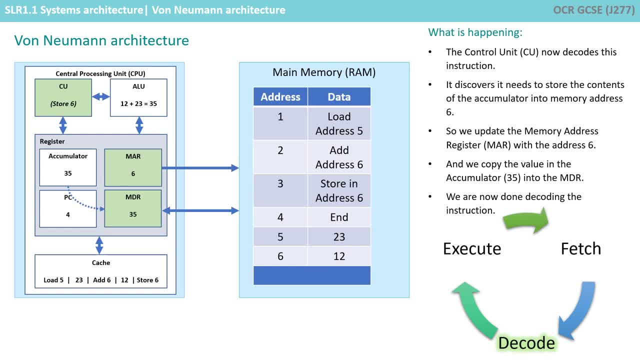 accumulator 35 into the MDR. We're now done decoding the instruction. We now execute the instruction, and so pass the address 6 down the address bus. We pass the value 35 down the data bus. This value ends up in address 6 and overwrites the contents which were there, which were 12.. 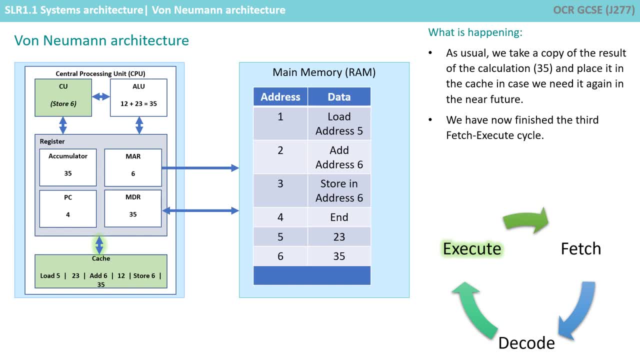 As usual, we take a copy of the result of the calculation 35 and place it in the cache in case we need it again in the future. OK, We've now finished the third fetch execute cycle. We're on our final fetch execute cycle. now and again, the program count is checked as: 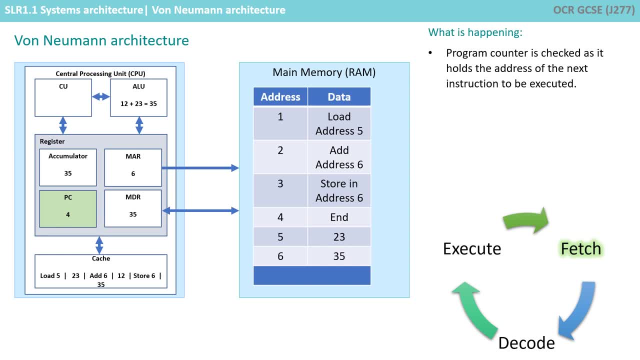 it holds the address of the next instruction to be executed. The address is copied into the memory address register. The address goes down the address bus. The contents held in address 4 are sent along the data bus and end up in the memory data register.